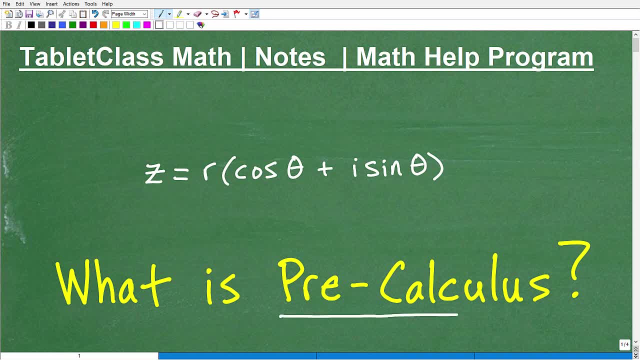 Okay, let's talk about pre-calculus, And pre-calculus is a pretty challenging course, And what we're looking at right here is some mathematical stuff. I'm just calling it stuff because I'm not going to explain this right now, But this is a mathematical things that you would 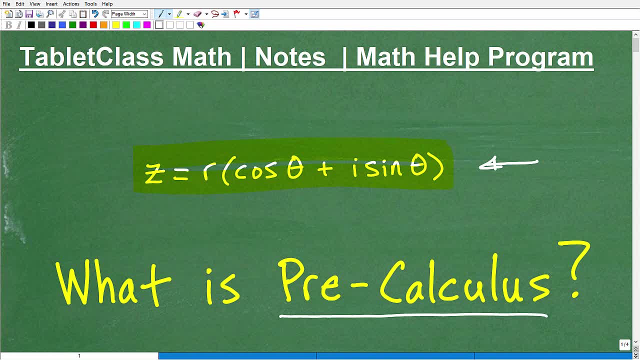 study in pre-calculus. Okay, And it's very. the name pre-calculus is very appropriate because you have to be successful and really understand all the topics in pre-calculus before you can really take on calculus. Okay, So if you have any intentions of, you know, going off to college, 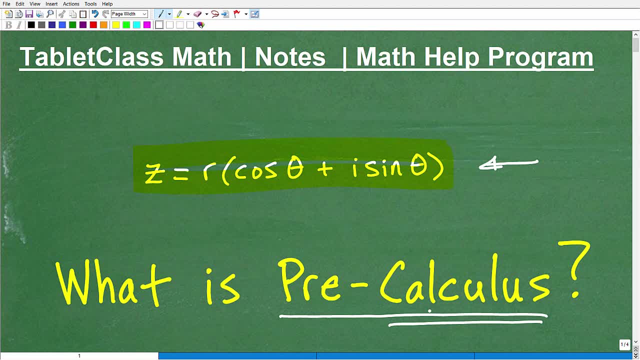 and doing anything, even it doesn't even have to be technical. You don't even have to be a engineer major or, you know, a computer science major, math major, whatnot. Even if you're a business major, finance major, you do have to take calculus We'll talk more about you know. 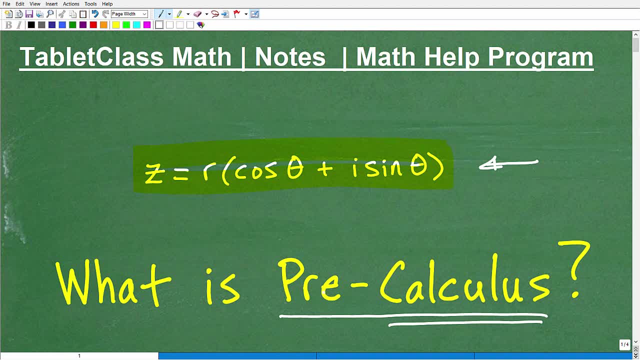 those of you who are considering should you take pre-calculus. I'm going to give you some suggestions on how to make that determination. We're also going to talk about when you should be taking pre-calculus. but I'm going to get into all of that in just one second. But to first quickly introduce myself, my name is. 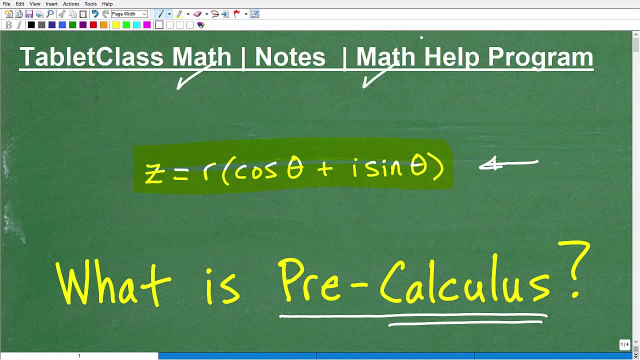 John. I'm the founder of Tablet Class Math. I'm also a middle and high school math teacher And over several years I've constructed what I'd like to believe is one of the best online math help programs there is. Now that's a pretty bold statement. I'll let you be the judge of that. If 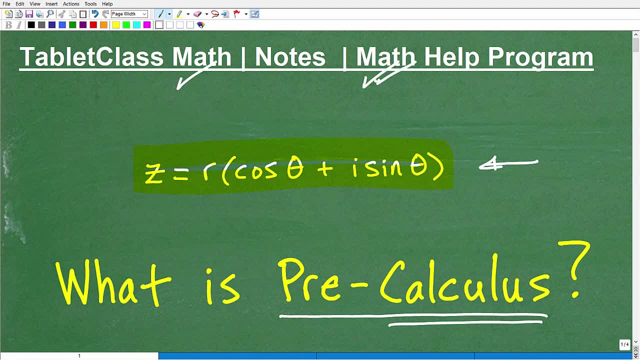 you're interested, you can check out my math help program Following the link in the description of this video. But basically I have one hundred plus different math courses, ranging from pre-algebra, algebra one, geometry, algebra two and pre-calculus. This is my most recent. 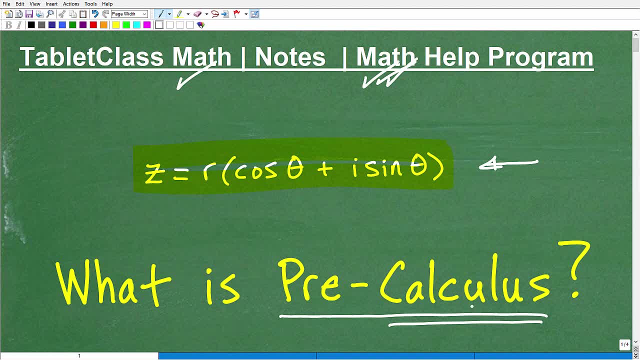 course, I just launched it, So that's why I'm kind of doing this video. But anyways, if you need help with pre-calculus, like immediate help, I'm going to leave the link- direct link- to my pre-calculus course in the 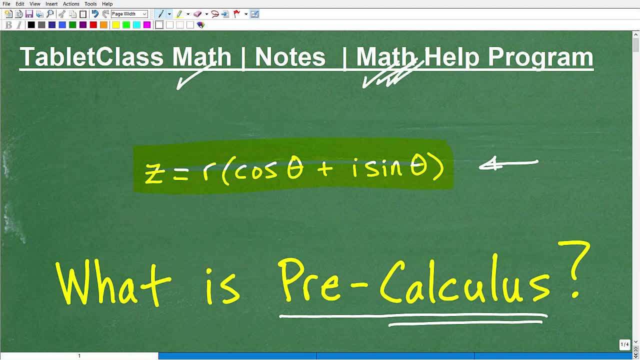 description of this video as well. But beyond that, I also have many courses in the area of test preparation. So if you're studying for the GED, HiSET, TASC, SAT, ACT, GRE, GMAT, ASVAB, ACCUPLACER, ALEKS exam, maybe a teacher certification exam and many, many others, I have great test prep courses. So just go to my website, check out my full course catalog. If I don't have what you are looking for, drop me a line and I'll help you out the best I can. I also do a lot with homeschooling, So if you homeschool, I have a great homeschool learning system. I've been working with homeschoolers for 15 plus years And last 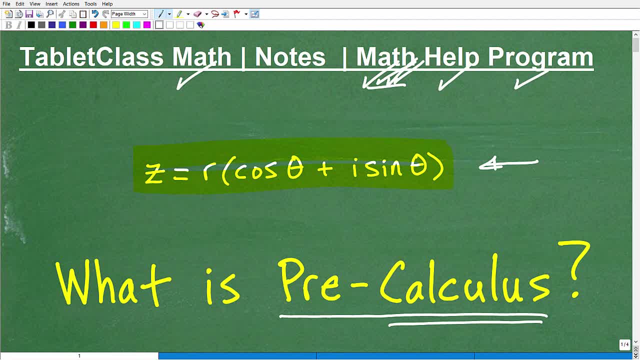 I helped those of you, obviously, that are having a tough time in your current math courses. Now, if you're truly serious about wanting to learn math and be great at math, then you got to be serious about your notes. Now, if you, you know, watch other videos of mine. you know I stress notes because you're here to know a little bit about math, But I always want to stress what it really takes to be a great math student. Okay, we'll talk about the specifics of this, But if you don't have this note taking business down, you're gonna have a tough time. you definitely won't be able to. 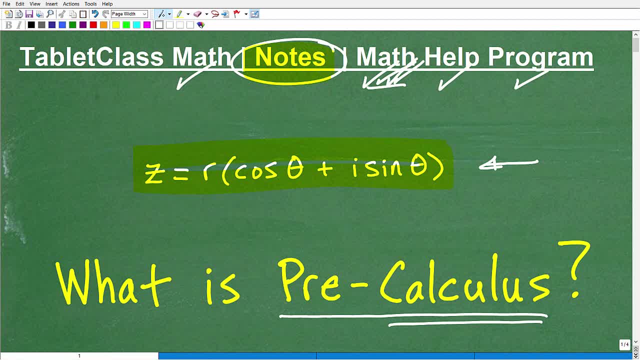 really pass pre calculus or any other kind of advanced math course. But bottom line is this: over decades of teaching math, it's apparent to me that those students who consistently take great math notes almost always do very well. And I would say that's an absolute requirement for anyone who's going to be taking pre calculus, because if you don't take great notes right, there's just too much information coming at you So you simply won't be able to, you know, to learn, keep up And typically poor. 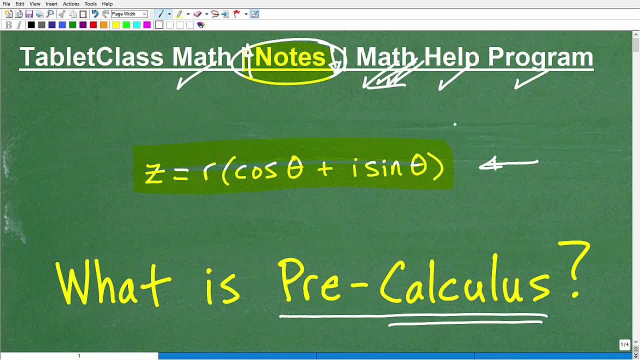 note taking, you know, starts off when you're in, like you know, elementary school, middle school and then kind of like in some basic high school courses, all the good stuff that I did way back in the good old 1980s. Believe me, I was not a great student because I wasn't really interested in school. You know, I went into Marine Corps, I did some other things in life And then finally, you know, after getting serious disciplined, you know, then I'm like: okay, you actually have to work to be a successful student, So you have to work on. 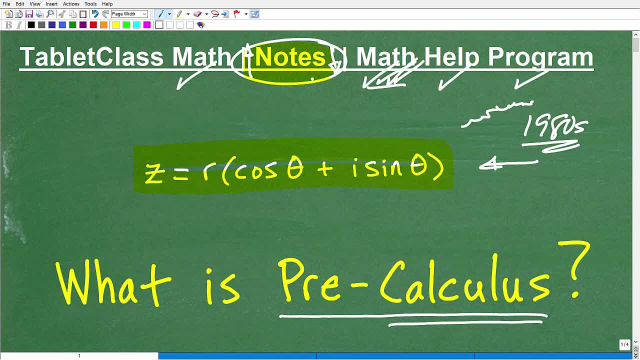 your notes. okay, put away the cell phone and engage with what the teacher is saying. write everything down and you're going to do very well. Now, in the meantime, as you're improving your notes, you can use my notes to study from. those would include pre algebra, algebra one, geometry, algebra two and trigonometry. you can find the links to those notes in the description of this video. Now, by the way, I am going to be working on creating a set of pre calculus notes, But if you are interested in pre calculus self for me, you definitely just want to go to my pre calculus. 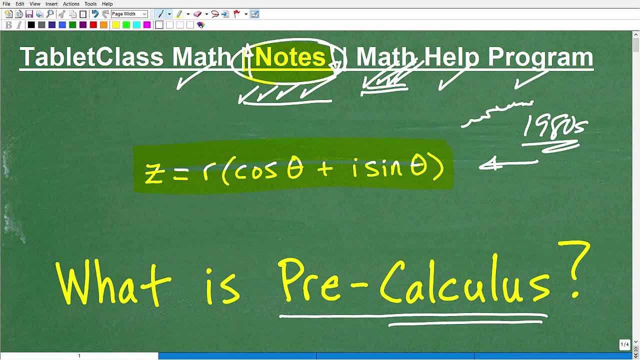 course, which again, I'll leave the link in the description of this video. So in pre calculus you get to learn all kinds of cool stuff like this. This is actually the trigonometric form of a complex number, And so some of you might be like: what is that? You're like, huh, trigonometric form of a complex number. Yes, You know, we have things like A plus B, I, and we can write it like this, And then we kind of do all kinds of crazy advanced stuff. This is necessary, You know. 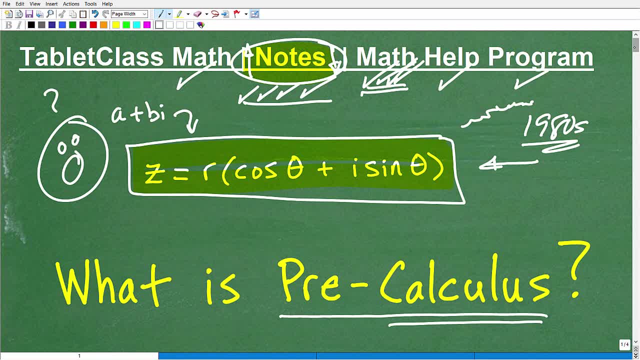 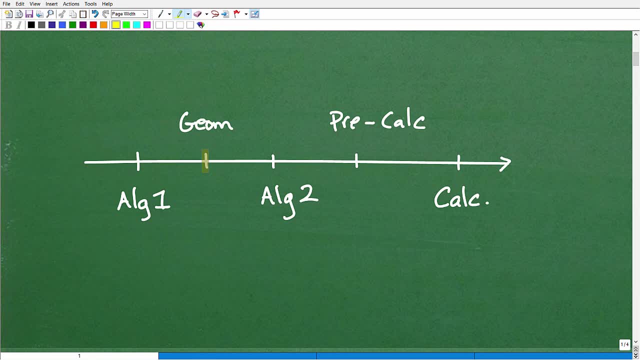 concepts and topics to be successful in calculus. Now let's take a look at kind of like a typical timeline for most students. So this is generally most people's high school. if you're kind of on a college prep track, it can. it can kind of change, But this is pretty typical. So you start off at your ninth grade year taking some sort of like algebra one course. Now again, this could be a little bit different than from what you have you're doing. And, by the way, over the last 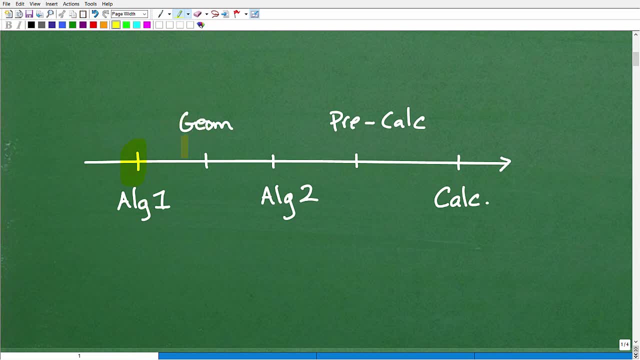 I would say 10 years plus. some schools have some curriculum, have combined algebra, one geometry. So if you haven't taken these courses, you know separately, like this, you're still getting the same information. Maybe that's the kind of better way for me to make this point. So you're going to learn your basic algebra, Of course, before that, in middle school, what have you taken? Well, you took pre algebra there again, but there's a course with the pre in it because you need to 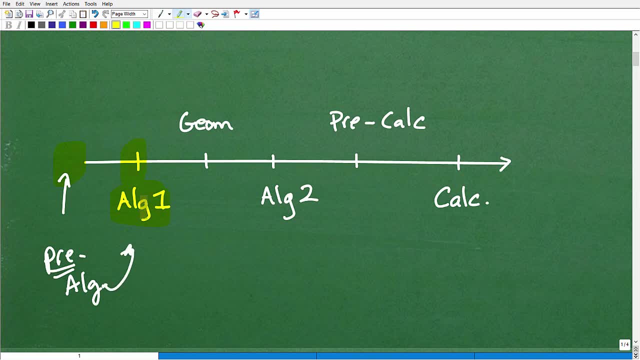 meet pre algebra to be successful in algebra one. Algebra one is very, very important course because it really is setting the foundation for college prep math. Then you got to go on and take a full year of high school level geometry And then you have to do algebra two. Okay, now for some of you that are curious about this, this is algebra two. other names of other courses are similar. algebra two could be like college algebra or intermediate algebra. This is typically like the community college version. 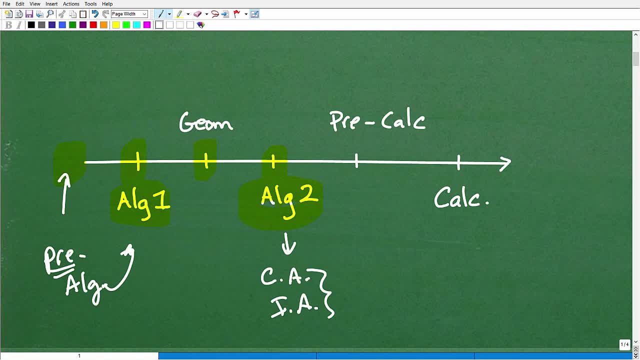 Of algebra two. sometimes I have a little trigonometry in here, But these, these courses are kind of closely aligned. Now, for most people, this is going to cover the majority of like, let's say, your high school graduation requirements. you don't even necessarily have to take algebra two. you could take other business course, general math, etc, etc. But if you're on a college prep track, okay, these are typically the courses you're going to be taking. now, for the most part, most students are going to be taking algebra two. 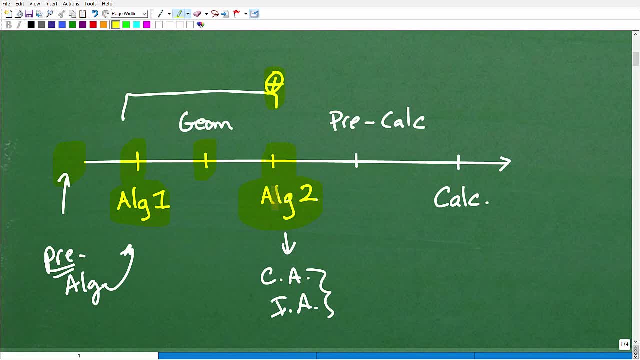 They're being in algebra two in their junior year. Okay, of course, again, there's always exceptions to this. That means that when you're a senior you have a choice. Okay, you can generally take like, let's say, a statistics stats class. right, You could see I should stick with math and not spelling, But you could take like a statistics course, which is an option. But I would say that the vast majority of people, students, should be taking pre calculus. Okay, especially. 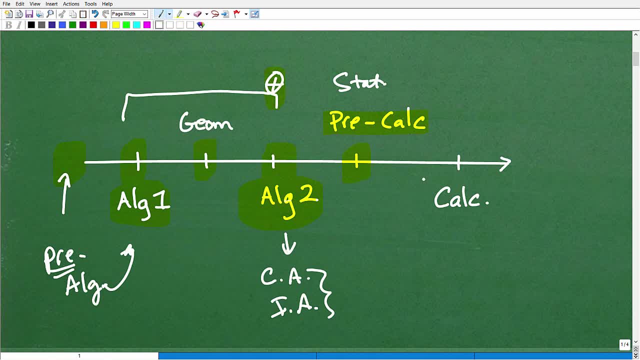 if you're college bound unless you absolutely know that you're not going to be, you know, business major or any kind of science technology kind of major in college. Okay, most of you should take pre calculus because you want to have that option open to take calculus as a freshman in college, Okay, so that's kind of the whole idea here. Now, some of you could be, some of you could take pre calculus and then go to school and not take any math. 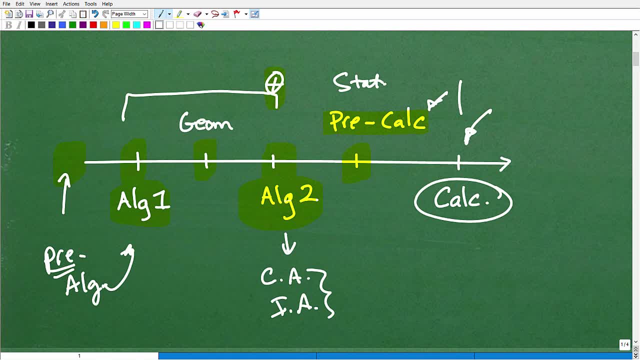 But you just kind of want to have that, as you know, just in case. that's fine too. But I mean, statistics is a great course as well, Okay, however, you can take statistics in college. But I really strongly suggest, if you're not sure you know which path you're going to go in in college and there's a chance that you'll, you know- do some sort of technical major, even business or finance majors, okay, you're going to have to take- for the most part you know- at least a semester. 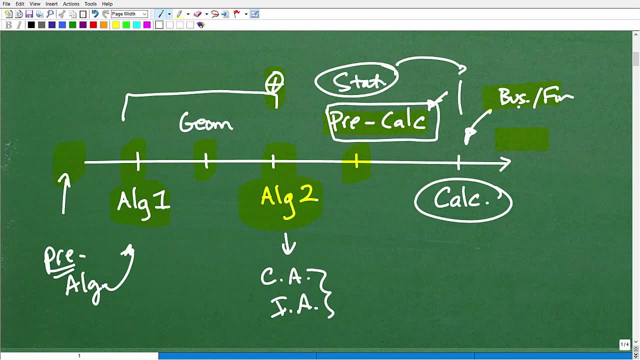 calculus. So don't close any options off, don't close any windows, majors, by not taking, let's say, pre calculus. I would just get this done If you have the chance to, in high school, if you're even considering college. it just opens up more windows for you because you're going to need pre calculus, obviously, to take calculus. Now, in college, calculus is typically broken up in like three semesters, So it's like calculus one, two. 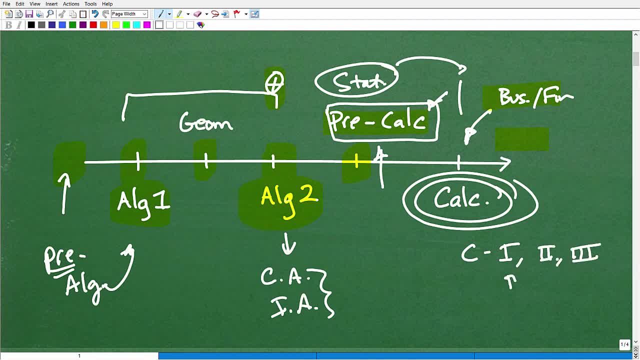 and three. So you have like single variable calculus, multivariable calculus and then, you know, get into more advanced calculus. So this would be like a year and a half worth of calculus. Now you could also be taking calculus as a senior in high school if you're doing calculus a, B, like your AP courses, which is excellent, which means that you were really accelerated. But the bottom line is this: you know we're focusing on pre calculus, So when should you take it? take it, you know I would obviously 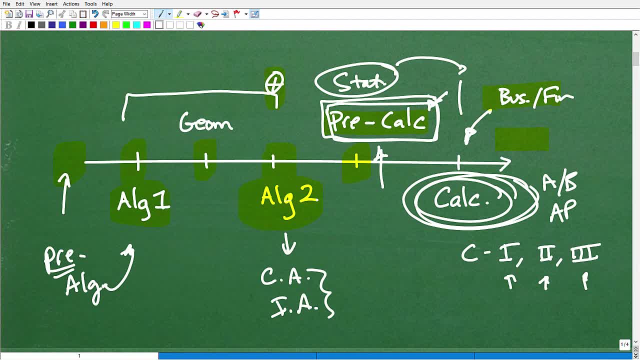 in high school. But you know, take it if you're. if there's even the slightest chance that you might do a technical major, okay, I would strong. and if you're not sure between pre calculus and statistics, I would take pre calculus, just in case. but this course is challenging, okay, even for the strongest of students, and you have to be very strong in algebra two. Now I'm going to get into the specifics of pre calculus here in a second, But let's talk about algebra one real fast. Okay, Now in algebra one. 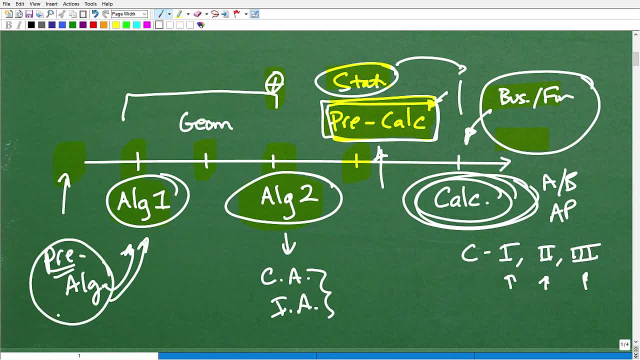 what happens? Well, you kind of relearn a lot of the stuff you learned in pre algebra and then you learn new stuff In algebra two. you kind of relearn all the stuff you learned in algebra one and then you learn new stuff In pre calculus. you're going to have to kind of really know algebra two really, really well And you're going to be learning a lot of new stuff. So now let's take a look at some of the topics here, And I state this because if you didn't do strong in algebra two, you're going to have a very difficult time in pre calculus. 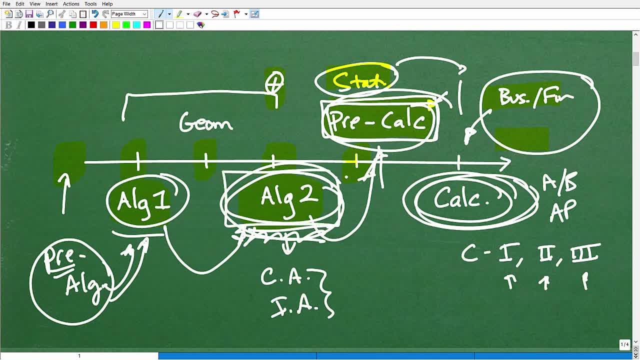 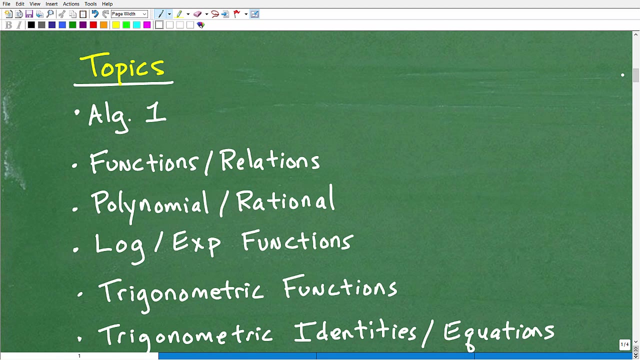 So if you are looking to take pre calculus next as your next course and you're struggling in algebra two, you got to get this right, okay, because if you, you know, finish algebra two in a kind of like unsure way, you're really going to be probably in trouble in pre calculus. So let's take a look at most pre calculus courses, how they look, the topics okay, and this is kind of off my course, And but again, most pre calculus courses are going to have these particular topics. 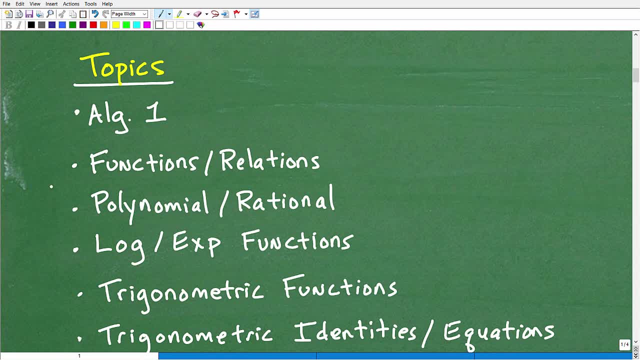 So let's go ahead and get into it. So this would be like your chapters, chapters 123, etc. So the first thing is, most pre calculus courses are going to start off with some sort of review- a couple weeks, maybe a month, and you're going to be reviewing a lot of different things from algebra one and algebra two, stuff that you should already know. okay, these are prerequisites, like you know: solving different type of equations, graphing linear equations, absolute value functions, all this kind of good stuff. So kind of like. 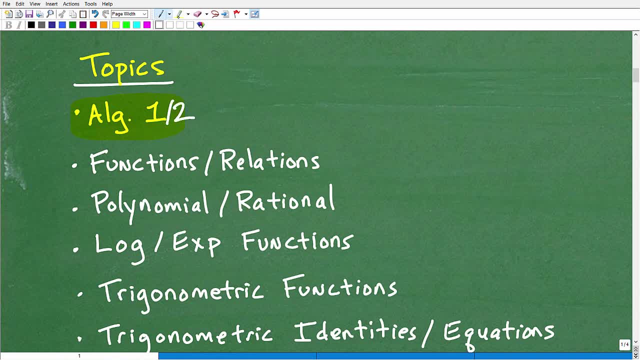 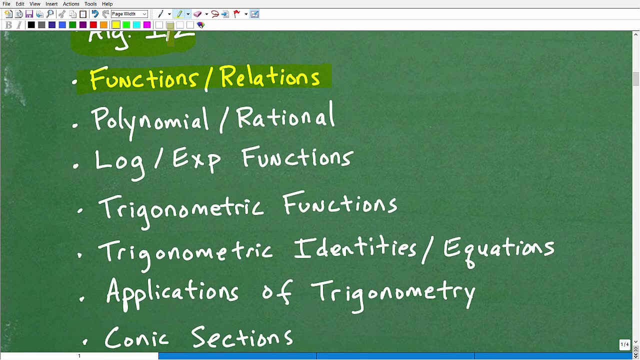 your algebra one. let's put an algebra two stuff as well, all right, all the things that you should really really have already mastered at this stage in the game. then you're going to have a chapter- again- this is most pre calculus courses, certainly mine- on functions and relations. Now, again, you should already know a lot about functions and relations, So you're going to cover the things that you should already know. plus, you're going to be learning more advanced stuff, especially when we're considering 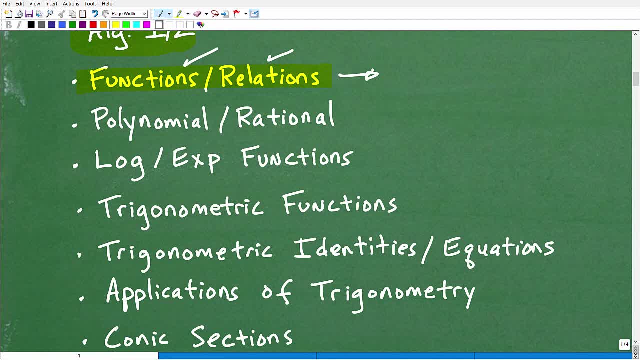 studying domain and range, symmetry, odd and even functions, etc. Some of the stuff that you haven't gotten in algebra one and algebra two. you're going to kind of extend your knowledge and functions and relations. Okay, Now, after that you'll typically take: there's a chapter on polynomial equations and rational functions- right, polynomial and rational functions- And this is going to cover all the stuff about polynomials again that you should already know, like solving quadratic equations. 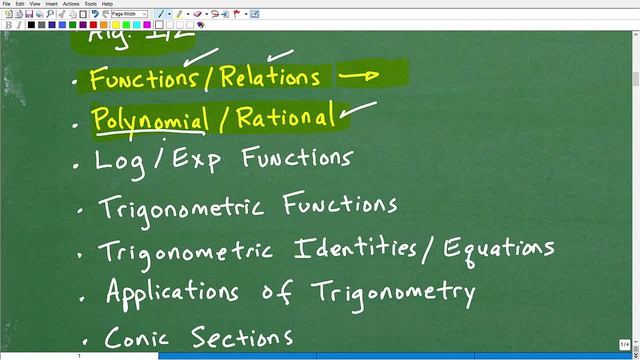 but some of the advanced stuff you were doing in algebra, two like long division, synthetic division, rational root theorem, Descartes, rules of signs, fundamental theorem of algebra. there's a lot of stuff that goes into. you know solving advanced polynomial equations, So you're going to get into. 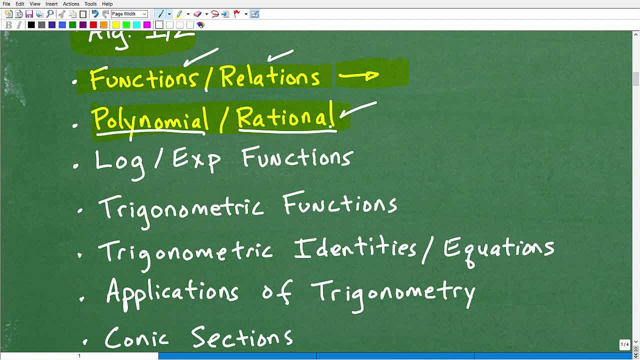 this again. And then, in terms of rational equations, you start, you know, covering a couple of things that you learned from algebra two: how to graph rational equations, how to equations and deal with, excuse me, rational inequalities. okay, this is something kind of. 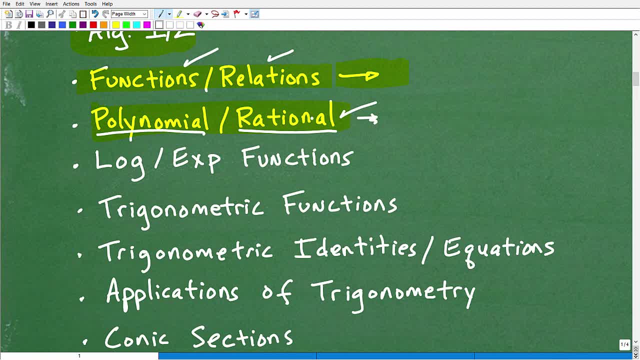 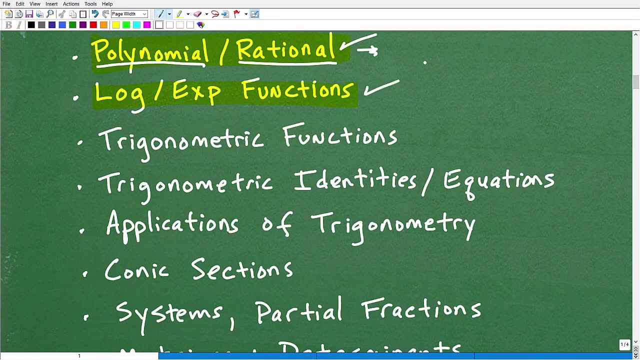 new rational inequalities. that typically is taught at the pre-calculus level. you might see some of these topics in algebra 2. all right, so moving on, you'll have a chapter on log rhythms and exponential functions. now, this should be a total rehash from stuff that you've done from algebra 2. 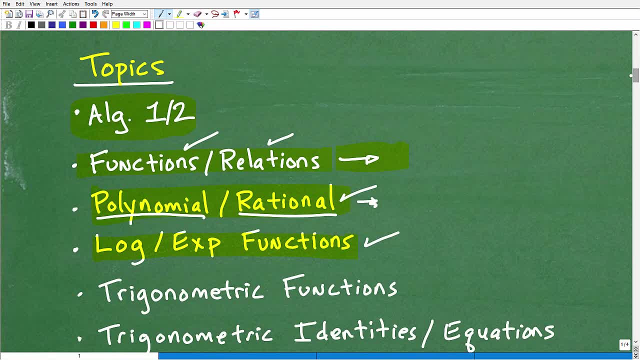 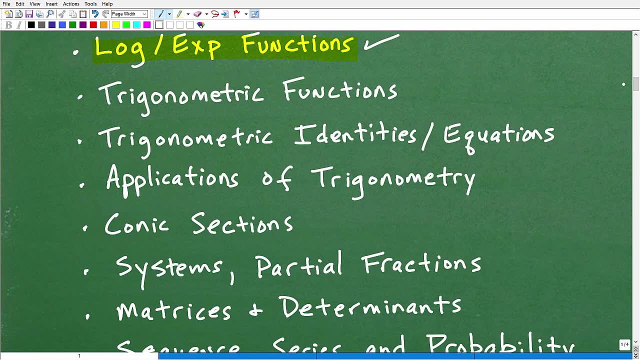 so a lot of this is going to be a review from algebra 2. okay, so if you did well in algebra 2, some of the stuff you'd be like, okay, i already know a lot of this and that is true. okay, all right. now, most pre-calculus courses break up trigonometry in about three chapters because 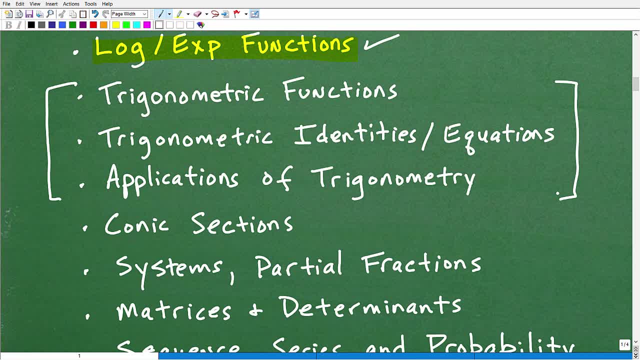 trigonometry is a huge part of pre-calculus and it's a pretty advanced part. so you'll have one chapter, typically on trigonometric functions. so this is all you know, your basic. you know how to work with sohcahtoa, but radians and how to evaluate trigonometric angles you do a lot of work without a calculator. you. 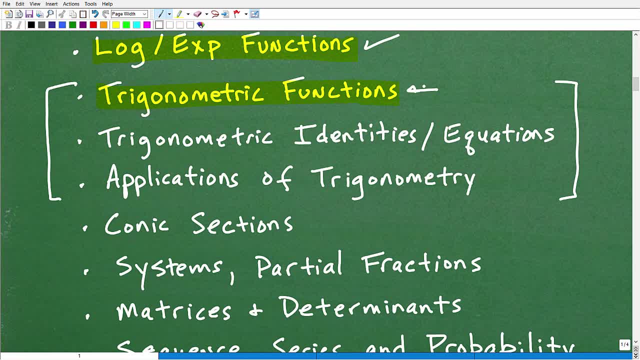 also get into how to graph sine and cosine and cosecant and secant. so this is this first chapter here. okay, there's still a lot to cover in this first chapter in trigonometry. then you get into another chapter on identities and equation: trigonometric identities and equations. 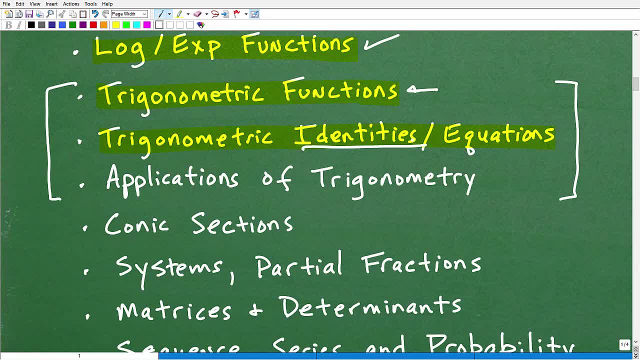 equations and there's a ton of identities and a lot of students typically don't like this when you're studying trigonometry, but it's very, very important. you need to know trigonometric identities. okay, there's double angle identities, half angles, sum of difference, product and sum fundamental. 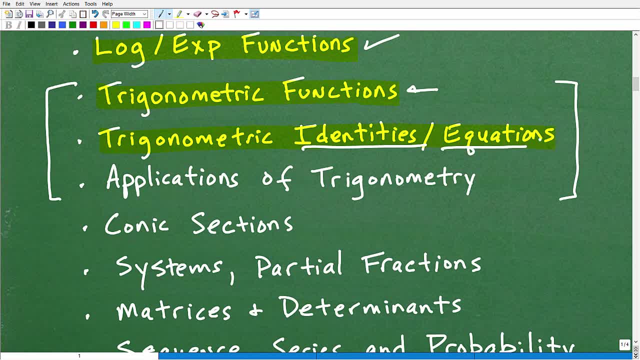 identities, and we're also going to learn how to solve trigonometric equations. okay, then you get into a chapter about the applications of trigonometry. so this is pretty advanced stuff as well. so this is kind of like this stuff. I was showing you in the beginning of this video how 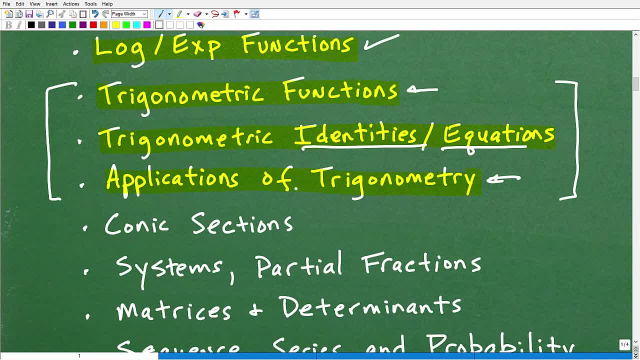 to. well, let's start off with like polar equations: how to write a complex number into trigonometric form so we can find the powers and roots of that. de morbes theorem, vectors, parametric equations, polar equations, how to graph this stuff. this is a very involved chapter as well, so you're going to. 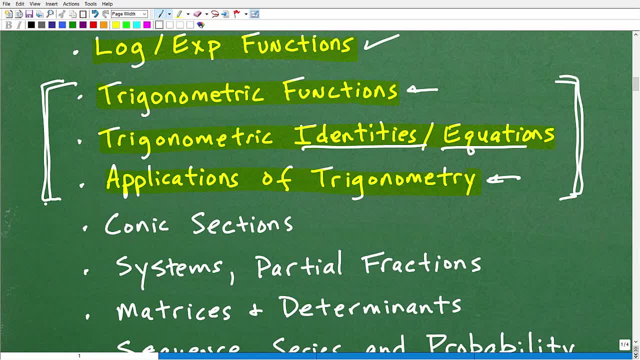 have three, at least three full chapters of trigonometry. okay, and it's going to be much more advanced trigonometry than what you're used to like basic. you know, SOH, CAH, TOA, kind of stuff. you know this is going to be far, far beyond that. 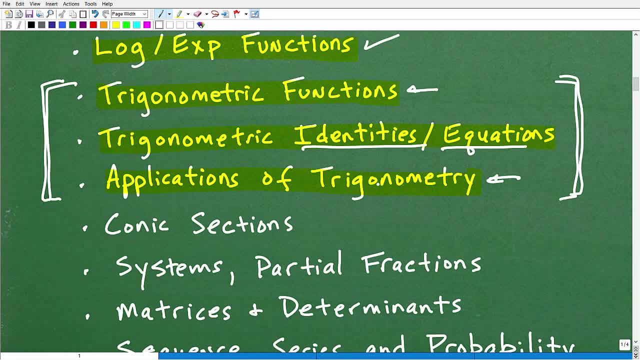 okay, and you need this stuff because in calculus there's quite a bit of trigonometry, working with a lot of different trigonometric functions, and you know, you got to know this stuff, all right. so I mean, let's take a look at what we've already looked at or like, wow, that's, that's a lot. well, we 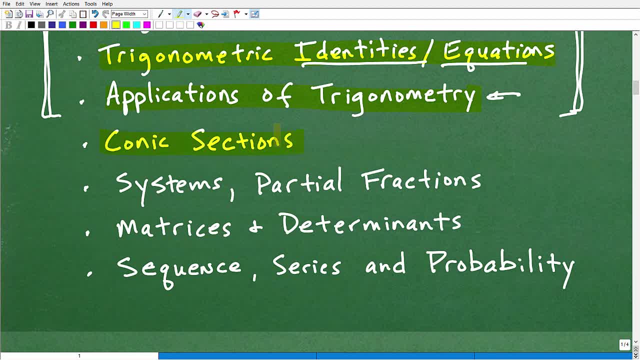 still have a lot more to cover. all right, so then you're going to get into analytic geometry, which we call conic sections. so this is going to be the study of like parabolas, um ellipses, um hyperbolas, um. let's see. what else do? we got here circles and then a translations of. 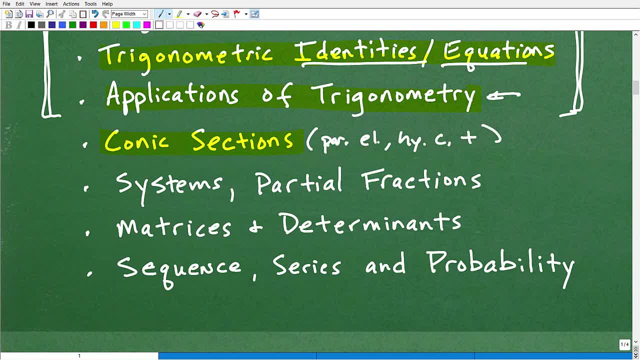 these guys. so this is a pretty involved chapter as well. and then you have another chapter on systems. now this is going to cover all the things that you should already know how to do, okay, how to solve two by two systems, all that kind of good stuff. but you get into more with systems. 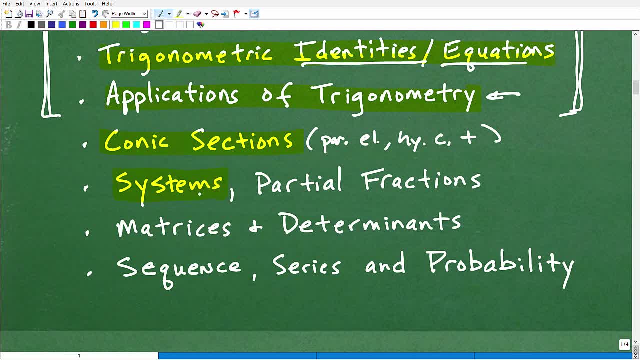 in this chapter you get into solving three variable systems, non-linear systems, and then, if you're lucky enough to have a course like mine that covers partial fractions, which I would say maybe half of pre-calculus courses cover, but this is very important as well, this is extremely well. 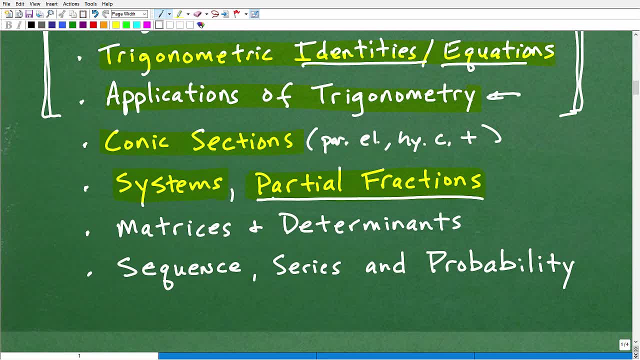 I got to watch my description here. this is very challenging, okay, partial fraction problems can be very difficult, but you need to know how to do partial fractions in calculus, okay, so anyway, you'll. that's typically within this chapter, so this is a lot of stuff you can see. you know, um, this is a challenging course, no doubt about it. all right, so after that you get. 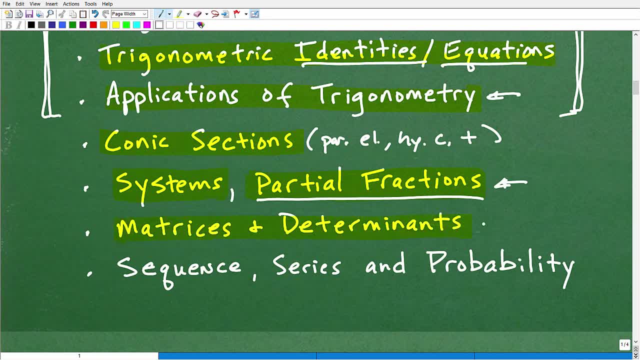 into another chapter on matrices and determinants. this should be a full, just a review of what you learned in Algebra 2: how to obviously multiply matrices, find the determinants of uh, of a three by three matrix, Kramer's rule, inverse matrices, Etc. so, or inverse Matrix, um. how to solve systems using a matrices, Etc. so again a. 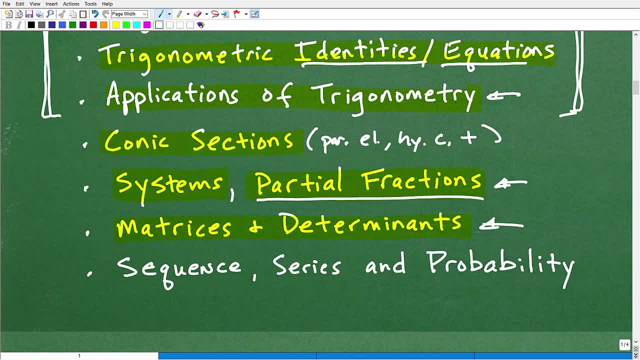 rehash. but you still, you know, um, you know need to cover this. just because you might have covered it in Algebra 2, like why do we have to cover it again? well, because, just like in pre-algebra and Algebra 1, you're kind of recovering, you're covering, you're building up, you know you kind of need to review. 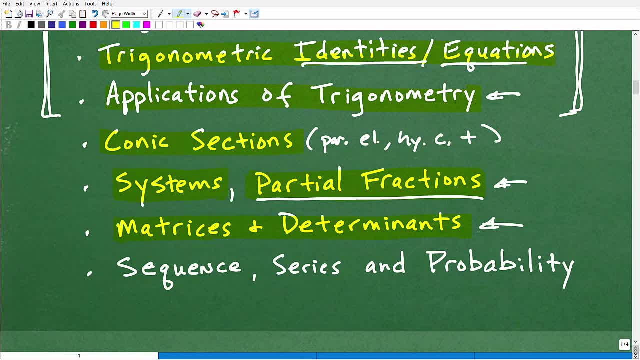 and strengthen your skills on this. all right, so let's talk about the last chapter. you're typically fine a pre-calculus course, and that would be on a sequence in series and probability. now, some of you may have touched on this in Algebra 2, but you're going to get it again in pre-calculus, so 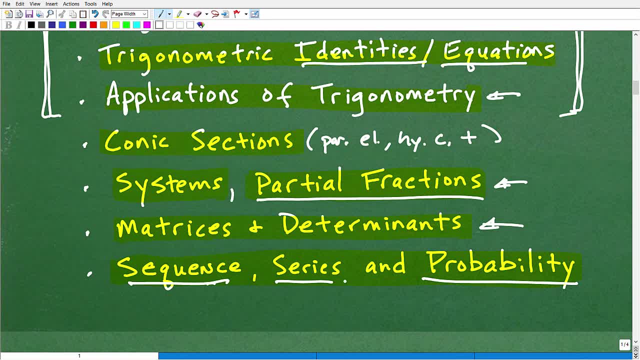 this is arithmetic and geometric sequence and series, infinite geometric series. let's see what else we got here. probability, this gets into, like combinations and permutations, and basic probability, etc. so this is a lot of stuff and, by the way, the binomial theorem is in here as well. now, a lot of. 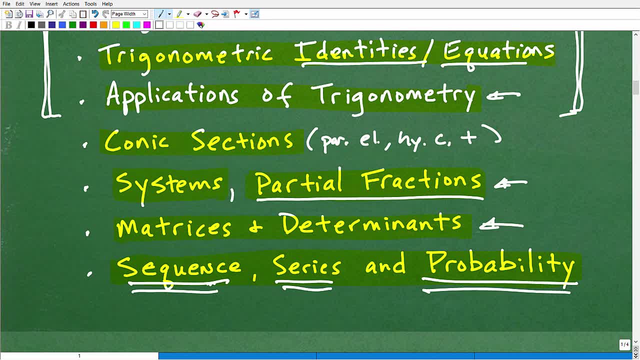 you out there. if you haven't taken pre-calculus, you have no idea what I'm talking about, right, because you haven't taken. well, you've taken some of this material like, okay, matrices and determinants. you probably may have taken some sequence in series. certainly have to have taken some systems. 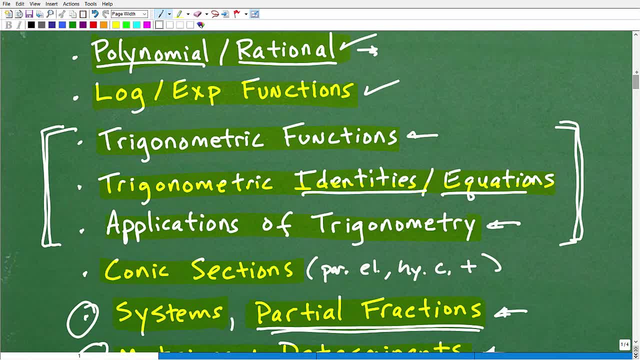 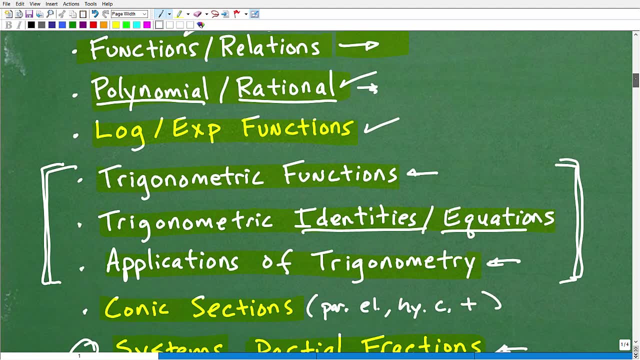 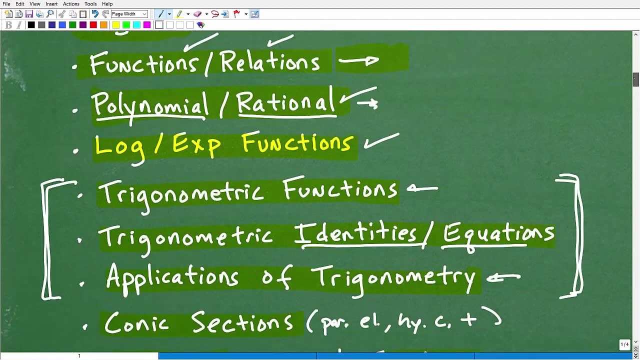 uh, but you don't know what partial fractions are, pretty sure conic sections. you might have taken some of that in algebra 2. but these are things that are going to help you for the rest of your life. so I hope you enjoyed that. be within your pre-calculus course. so this is a lot, okay. every chapter is pretty challenging, okay. 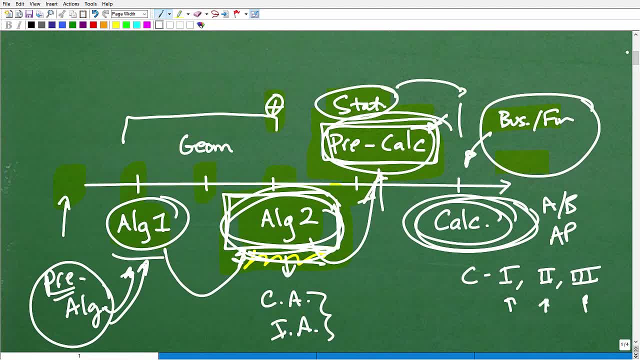 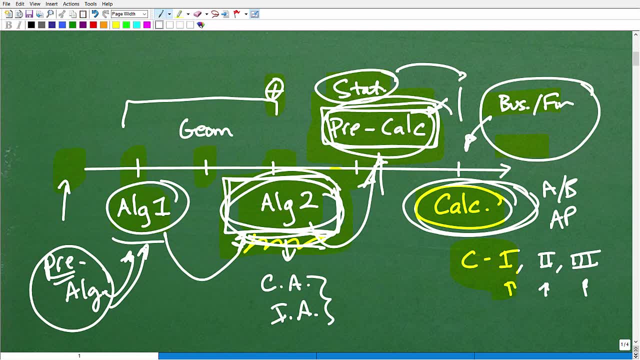 but you need to take this, all right when you go on to calculus in college. all right, this is coming at you. you know big time right, and i, you know, even the strongest of students uh, can get quickly overwhelmed. uh, you know taking calculus because they're not ready for it. okay, so again, if you, you, 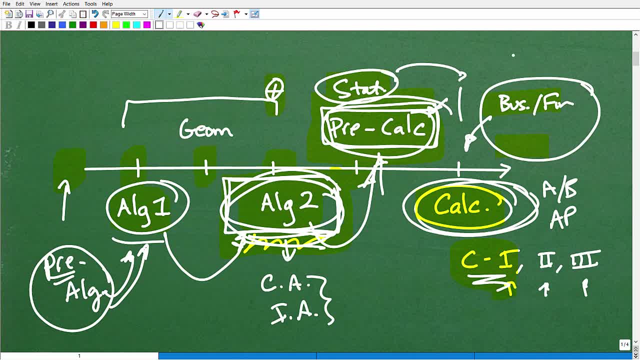 have to be strategic about where you're going in life. if you're going to college and if you want to consider majors, that may involve you taking a more advanced math course, okay, you need to start thinking about that in high school. all right, you have to be thinking about. all right, what do i got? 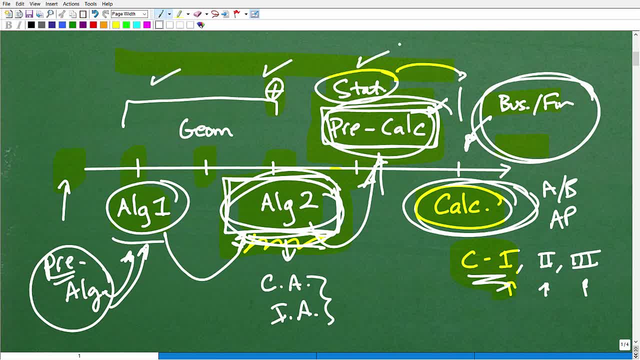 to be doing well. you got to be building up your math skills one step at a time. okay, because you're not going to do well in algebra 2 if you haven't done reasonably well in algebra 1. but here's the thing, there's always hope, right? so even if you struggle in algebra 2 and you have to, 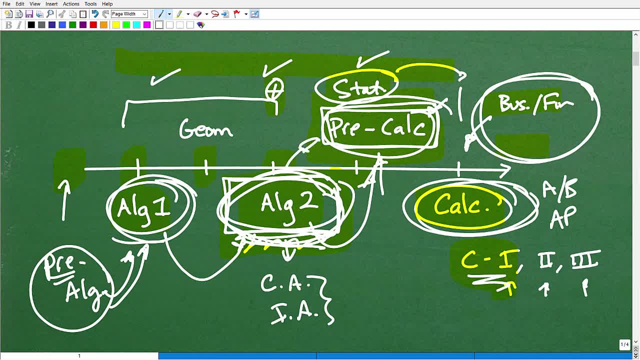 take pre-calculus or you're looking to take it? what? what do you have to do? well, you have to get better at math. you're going to have to go back and do some review, and there's a number of different ways you can do that. you can um get with your teacher and ask what they think, but probably the 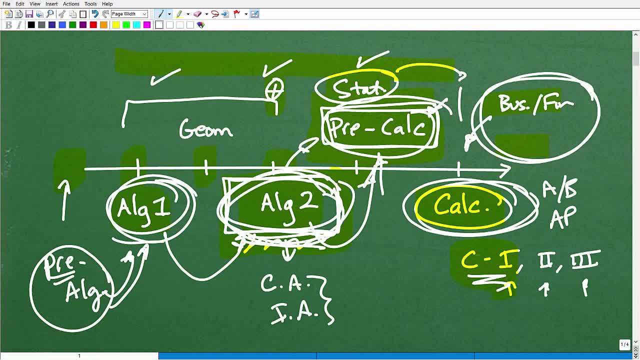 best way is to maybe use a program like mine. uh, you know, take a look at my algebra 2 course, review it independently, take some initiative, you know, especially if you are in between, let's say a summer break, if you're taking pre-calculus and you have the summer, you know, to kind of get ready for it. i 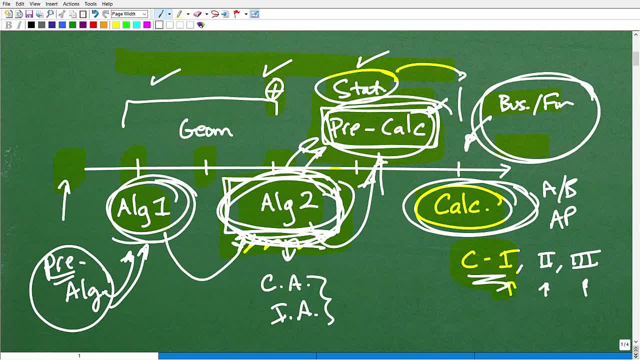 would say: definitely take advantage. okay, um, do things that you don't have to do, take the initiative and you can get yourself caught up, right. but if you just kind of rely on, well, all right, i wasn't that strong in algebra 2, but i'll just kind of relearn it. 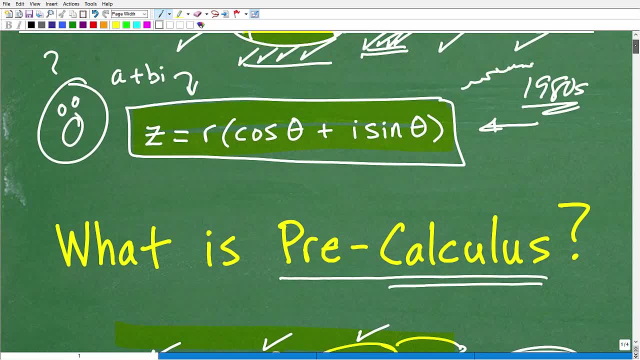 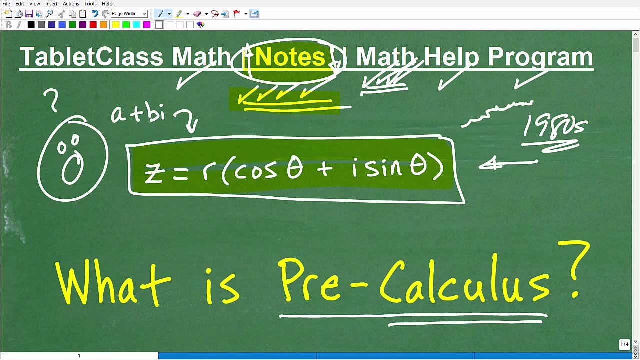 by taking the course. well, that's a pretty big risk. okay, and certainly if you're not, you know over the. you know strong academically in terms of your habits, strong note takers, study hard, do all the homework, etc, etc. you may end up looking like this: all right, uh, because you know pre-calculus, there's. 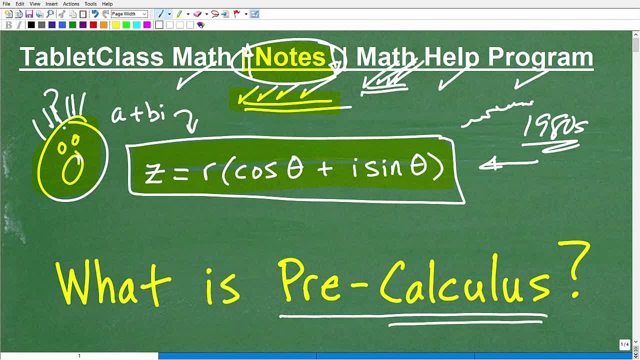 some. there's some topics in here that you know that will just make even the stronger students go like: ah, i have no idea, but listen, you know. uh, people have done this throughout. you know millions of people have taken pre-calculus successfully that probably thought that they couldn't, so you. 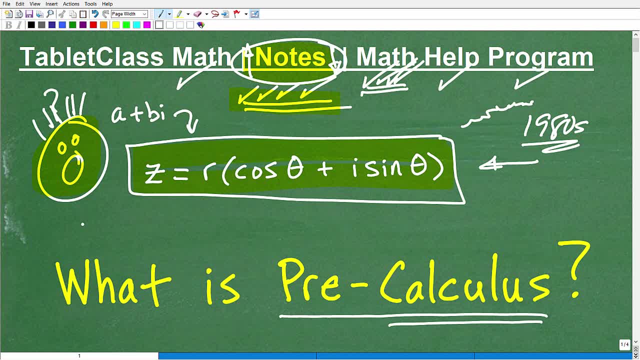 can do it as well, but it you know, it is a course that uh requires respect. okay, in terms of don't underestimate how challenging pre-calculus can, be okay, but it's extremely important, um, as all the reasons we talked about, all right. so, um, if you need help with pre-calculus, 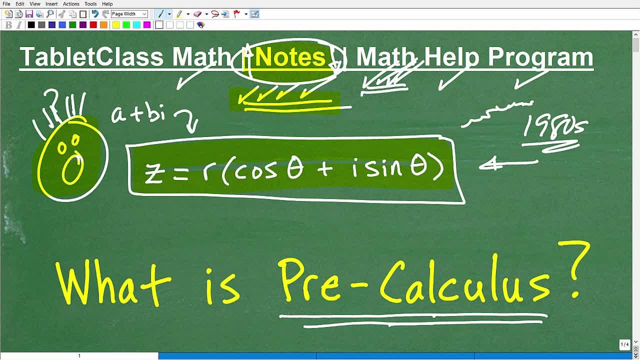 okay, i post a lot of advanced material on my youtube channel, so you might want to consider subscribing. and, by the way, if you like this video in some small way, please consider smashing the like button. but, um, as i post more advanced material, you know, like pre-calculus level, 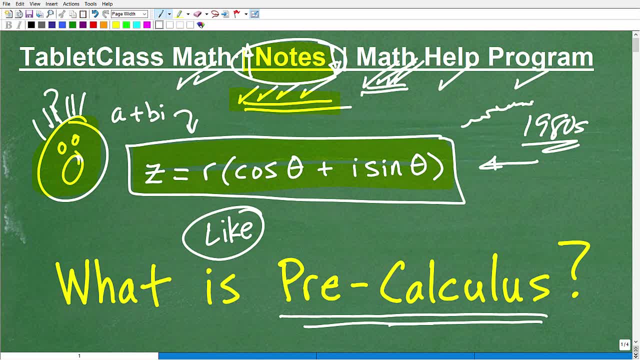 material. you're gonna need more help than that. so i would strongly suggest maybe checking out my pre-calculus course or looking for it's something else. okay, above and beyond um, you know maybe what your your current course offers, okay, but if you're in pre-calculus right now, 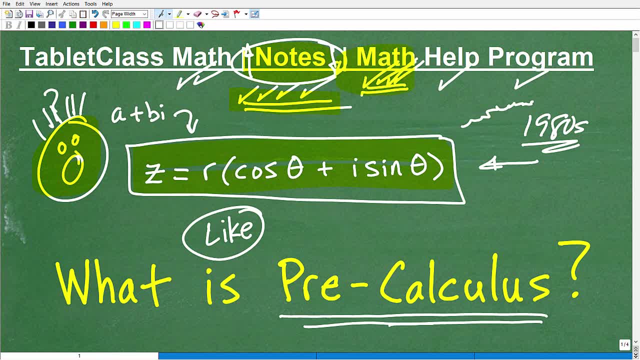 you definitely need to be talking to your teacher. all right, be like: hey, teacher, help me out, what do i need to do? that's your first line of you. know the defense against a poor grade, right, Like, take great notes, go on the initiative, talk to your